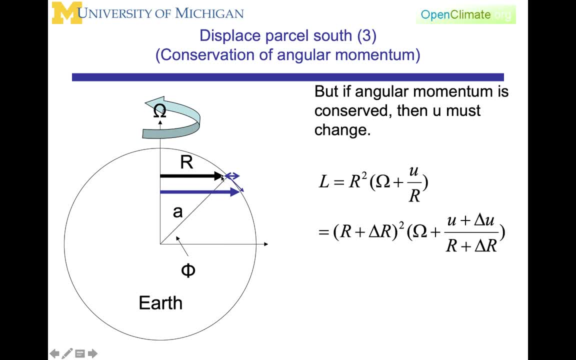 What we want to do now is to consider the angular momentum at these two places. So the angular momentum per unit mass is going to be r, squared times big omega, plus u over r. If we're moving to this new place, then L here is going to be r plus delta, r, squared times in parentheses, the large omega, and there's going to be u plus delta, u and r plus delta, r, closed parentheses here. 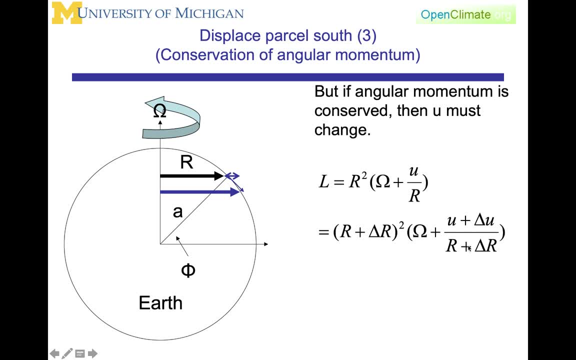 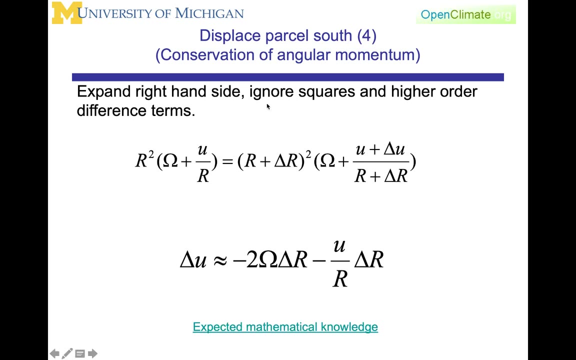 So this is the relative angular momentum per unit mass at the new location. If it's conserved, then what we're going to say is that the angular momentum in these two locations is equal. We're going to expand the right-hand side and ignore the squares and the higher-order terms. 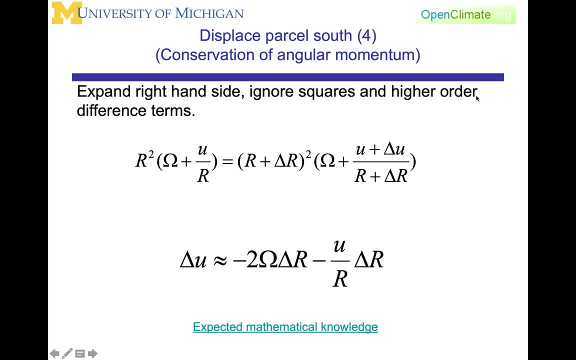 Again, we're going to expand the right-hand side, ignore the squares and the higher-order terms. If this does not make sense to you, then you need to go back and review the expected mathematical knowledge in the course And we're going to end up with a delta u- a change in velocity is going to be approximately. 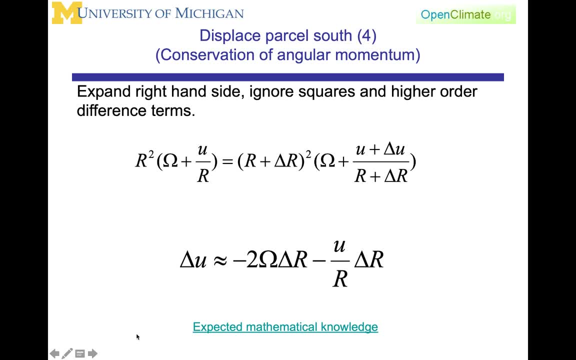 and the approximation comes from where. ignoring squares and higher-order terms, It's going to be approximately minus 2 omega delta r, minus u over r delta r. So we have related u to the change in the radius of rotation around the axis. We've related u to that change in such a way that this equation remains true. 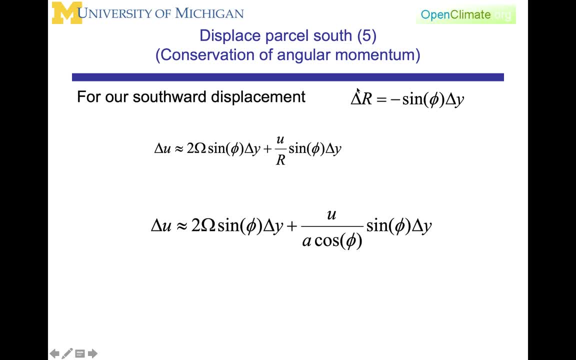 For our southward displacement. we can then calculate that delta r is equal to minus the sine of the latitude times, delta y. So we go back to our original displacement of delta y And then, making that substitute, we can relate delta u, the change in the relative velocity to the displacement, delta y. 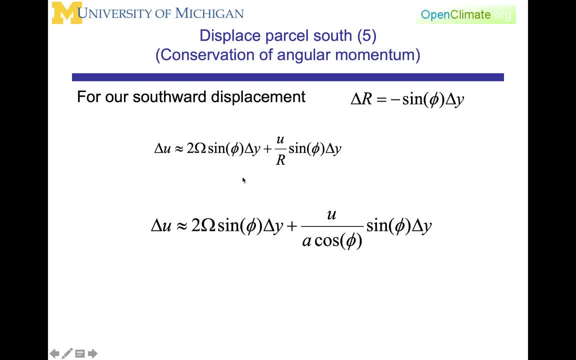 And it's going to be 2 omega sine of the latitude delta y plus u over r sine of the latitude delta y, Hence delta u. the change in velocity is going to be approximately 2 omega sine latitude delta y plus u over a cosine latitude delta y. 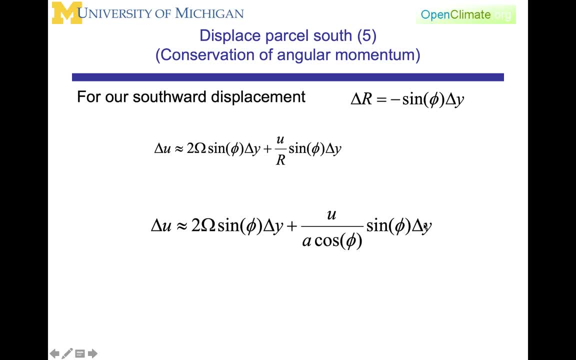 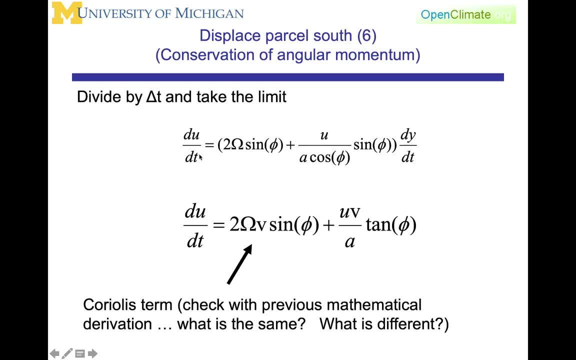 Where- here we have just simply used the definition of a cosine- latitude is equal to r to r. If we divide by delta t and then take the limit as delta t and delta y go to zero, then we see that du dt- the acceleration that has occurred due to this displacement- is going to be two omega. 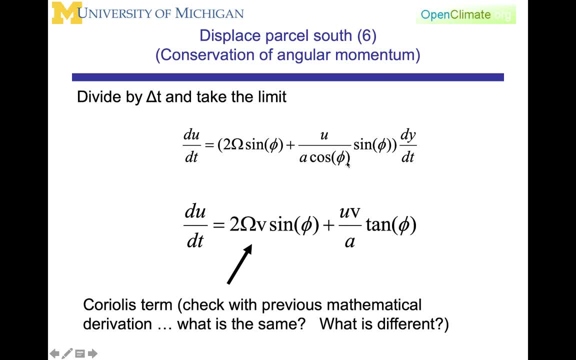 sine latitude plus u over a cosine latitude sine latitude, times a dy, dt here. and we are going to recognize from our previous consideration in the rotating coordinate system that this two Omega V sine of latitude is the Coriolis term and I invite you to check with the derivation. 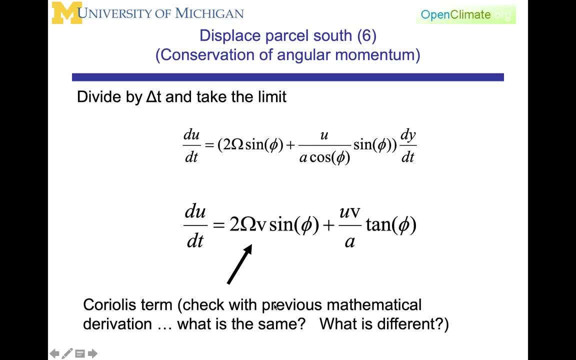 that we did in the rotating coordinate system lecture, to see what is the same and what is different from the form of these two equations. we've also used the definition of the derivative here, that the sine over cosine is equal to the tangent and that dy dt is equal to V. so we see 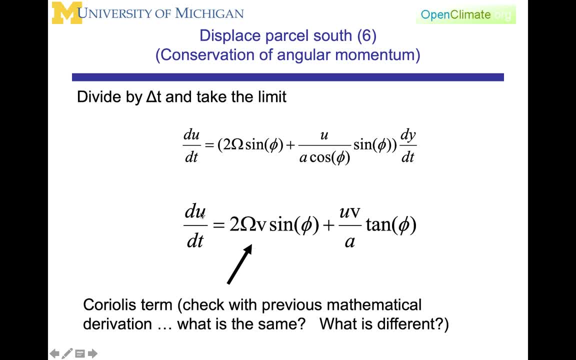 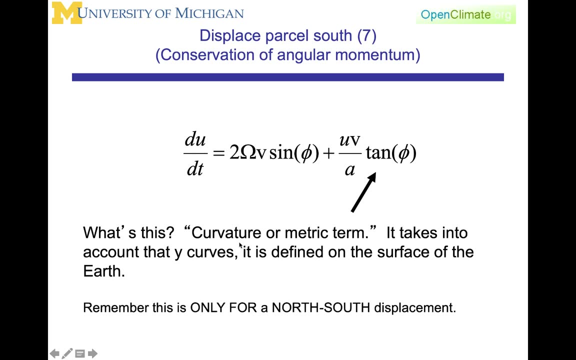 this relationship, that the acceleration in the x direction or the longitudinal direction is going to be related to the velocity in the y direction or the latitudinal direction. what is this term? what's this additional term that's sitting out here? uv over a tangent, and this is one of the terms that is called the curvature of the metric term. 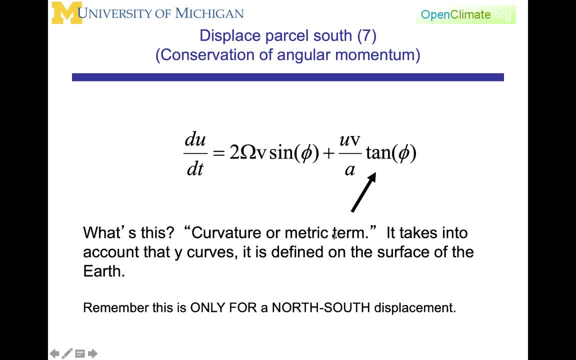 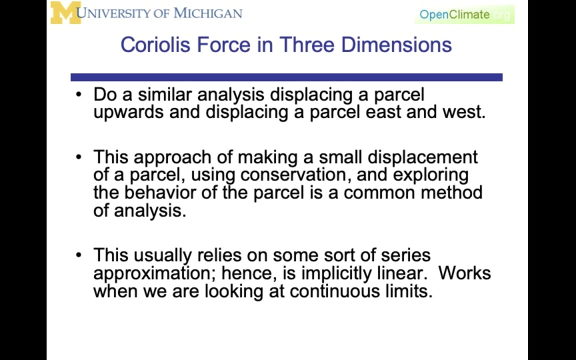 and it takes into account that why that displacement actually curves is defined on the surface of the earth. you should remember that what we have done here is only for a displacement in the north-south direction, and if we were to repeat this with a displacement in the east-west direction, then we can follow the derivation in the Holton. 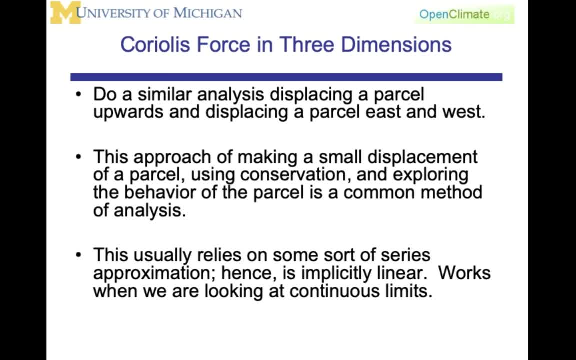 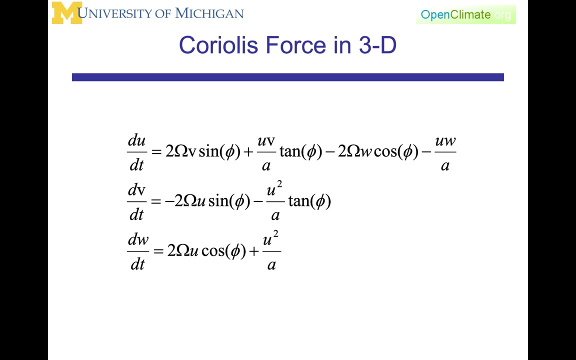 and Hakeem textbook, and using conservation and relying on some sort of series approximations. this is a explicitly linear derivation. if we do this similar analysis in three dimensions, we can get this representation of what we might call a combination of the Coriolis term and the curvature or the 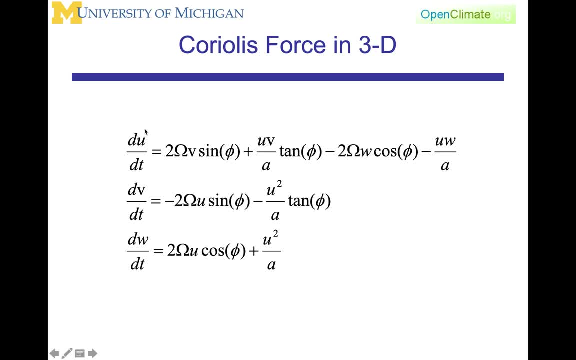 metric terms in three dimensions. The acceleration in the u direction or the acceleration in the x direction is proportional to the velocity in the y direction. We also see here a term that's related to w, the vertical velocity. Here in the meridional direction, we see that the acceleration in the 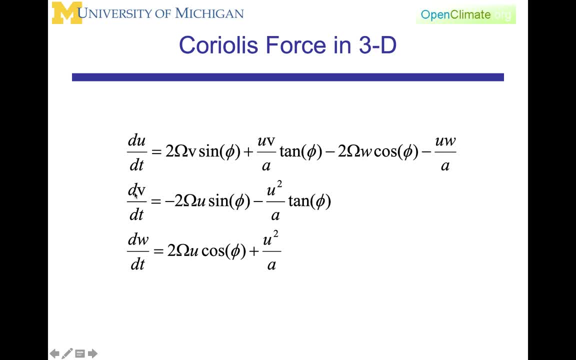 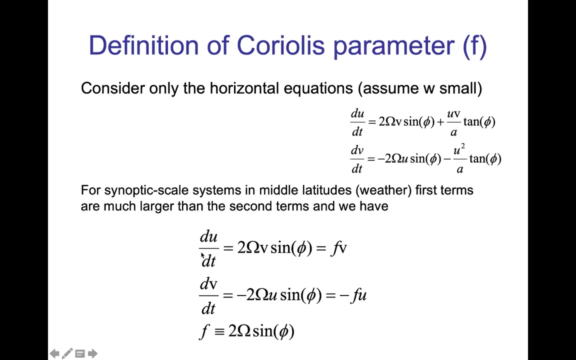 v or the y or the meridional direction is related to the velocity in the zonal or the x direction, and we see a vertical term where the acceleration in the vertical is proportional also to the velocity in another direction, and here in the u direction, If we consider only the horizontal. 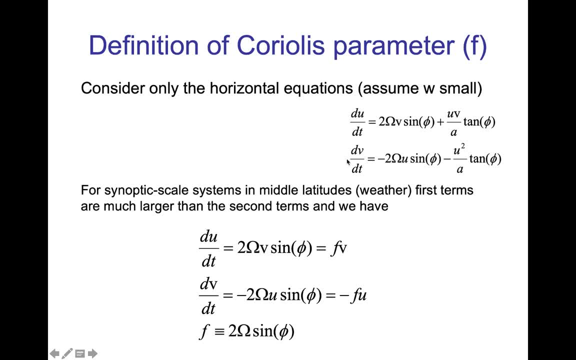 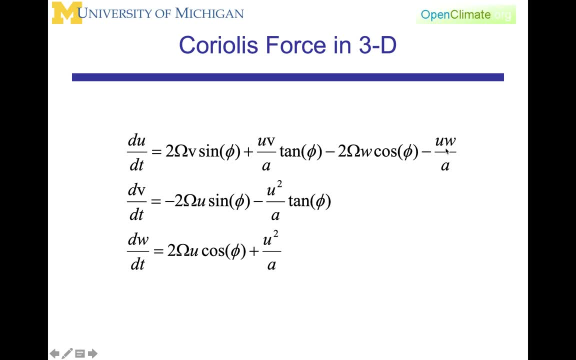 equations: assumed that w is small, then the w that was in this preceding slide. here and here we have made the decision that we can ignore them. so this is an approximation that you may have to come back and revisit at some time in the future. With the assumption that w is small, then the equations: 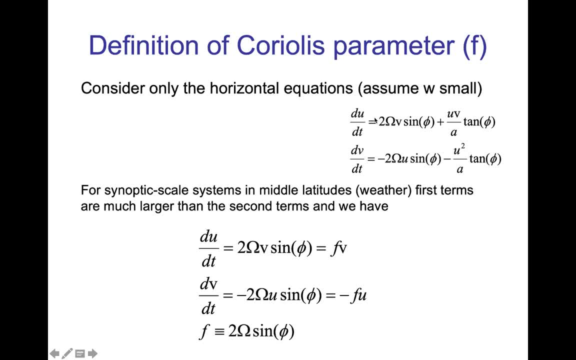 on the preceding slide, reduced to this form, where we have a term that looks like the Coriolis term and a term that looks like the meridional direction. If we consider only the horizontal equation in the $24-ader muss strings, we will know that it's one-third miss angelic by 0.54. 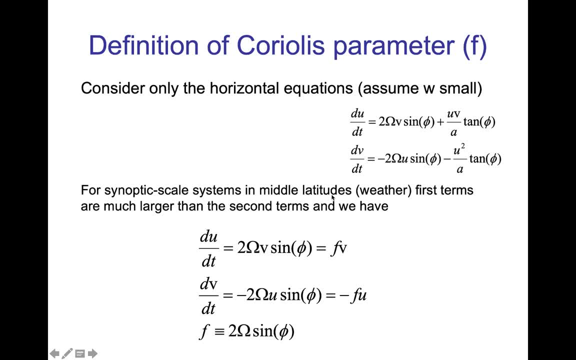 as it falls below that of the original result of w. so k was ten moreawrds out of the v $24-ader muss term. we will see anything different here. There's three scenarios here. which looks like w called the curvature of the metric terms For synoptic scale systems in mid latitudes, the 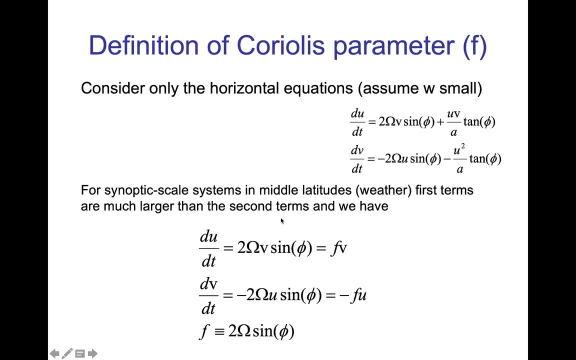 first terms these drawings were pretty strong for you to read out for great ease. other point you may as well understand- it's a fairly quick process to here are much larger than the second terms. so again we have made an implicit profes saptAlQuery nt t stronger than the Ww. Demonst cualities professor.